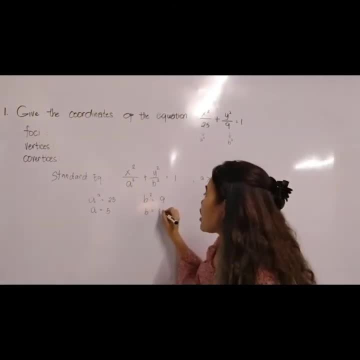 b. this square root of 9 is 3.. Okay, so this is a and b. Let's get this. How much is the purpose of this formula? okay, Let's calculate the total amount of b squared. So what's the? 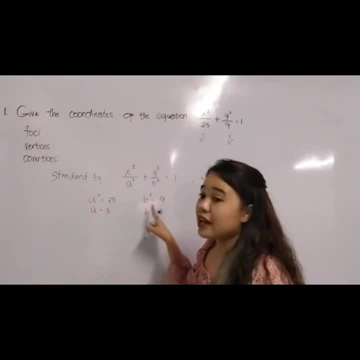 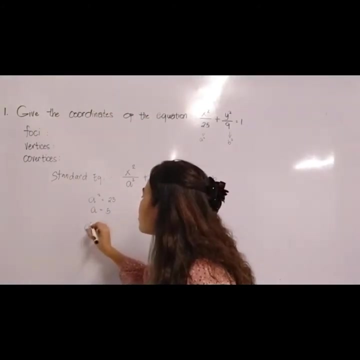 we can see the value of a and b. the most important, or one of the most important variable in order to graph our ellipse, is the value of c. okay, c is just equal to in our previous discussion. c is equal to the square root of. 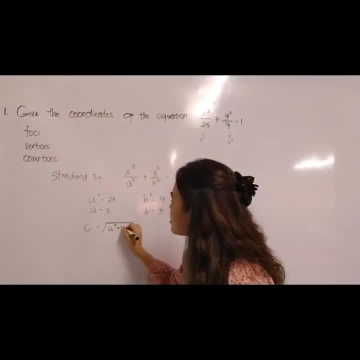 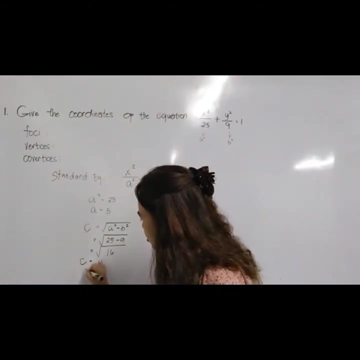 k squared minus b squared: okay. so this is 25 minus 9, which is 25 minus 9 is okay. that is 16, which is square root of 16 is 4, so the value of c is 4. okay, now we already. 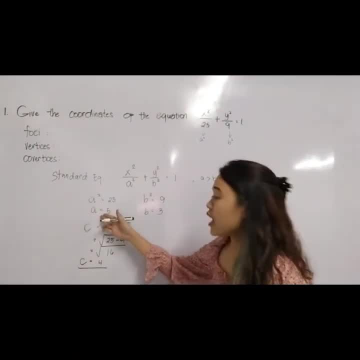 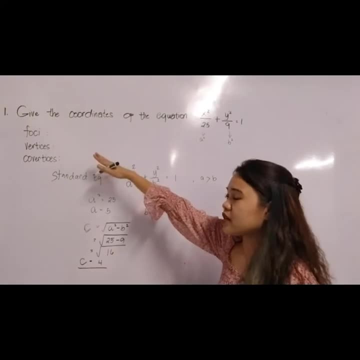 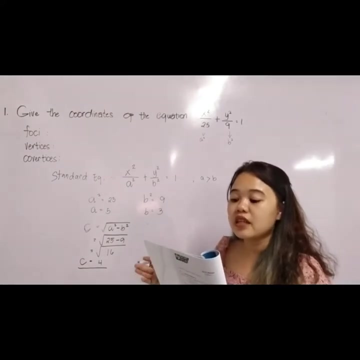 have the value of c, which is 4, a, 5 and b, which is 3. can we now find our coordinates of the foci? let's read the definition of a foci. each focus is c units away from the center. so the value of c is 4. 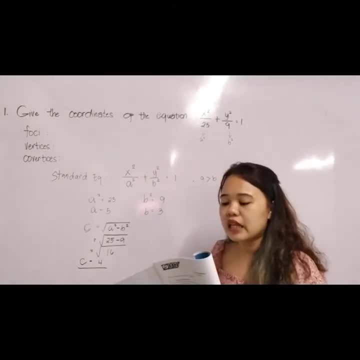 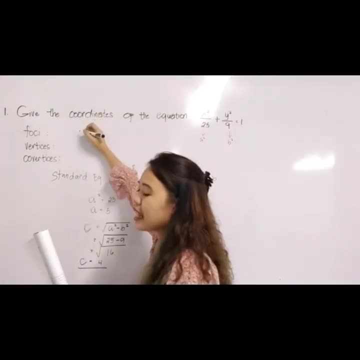 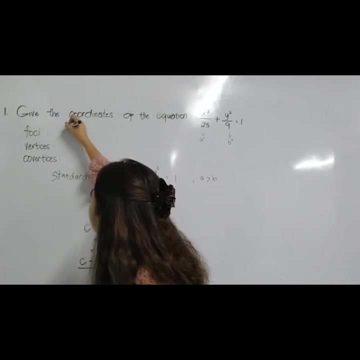 units away from the center. for any point of the ellipse, the sum of its distances from the foci is 2 to the 8th, so f1 can be written as negative. c again, this is um. wait, I don't have a marker. f1 is negative. 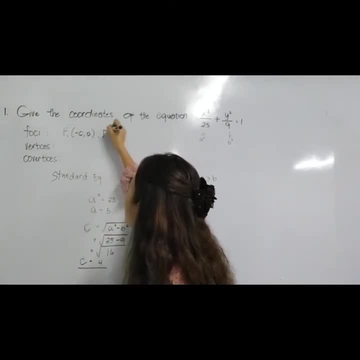 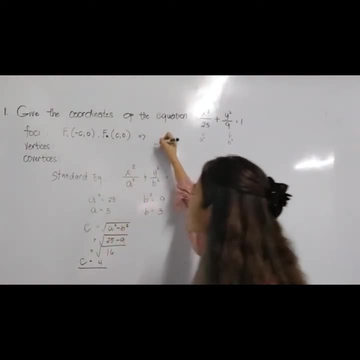 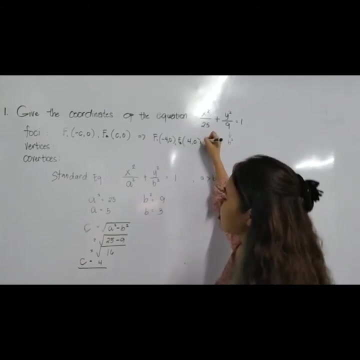 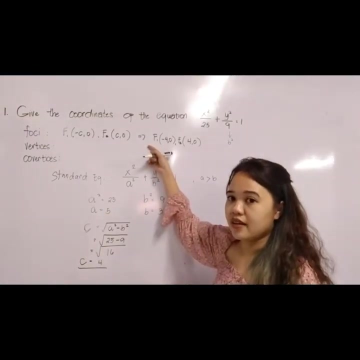 c 0 and f2 is c 0, okay, so that's why we have f1 as negative 4 0 and f2, which is we have positive 4 0, okay, those are our foci. okay, so f1 and f2. 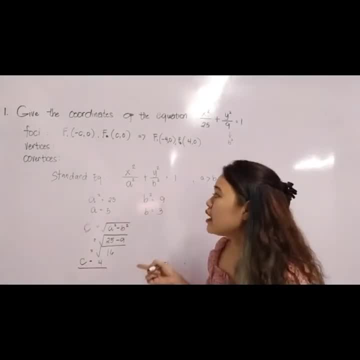 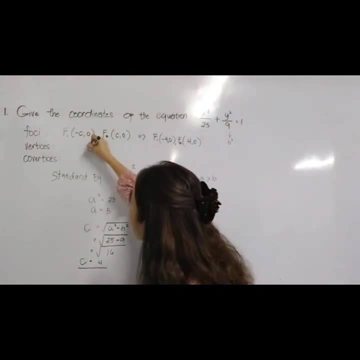 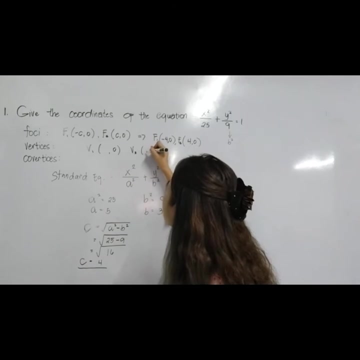 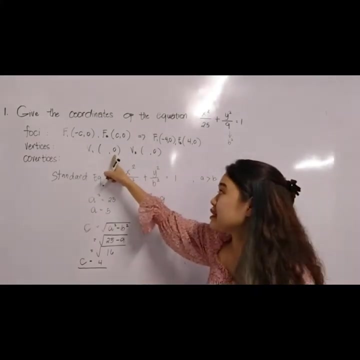 next is our vertices. our vertices if our value of y is 0. so if this is 0, then we have v1. if our y is 0, v2 again. if our y is 0, then the value of x is equal to positive and negative. 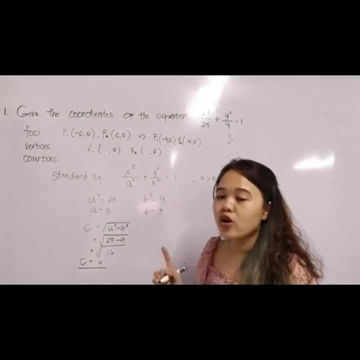 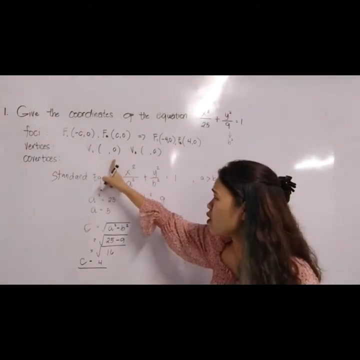 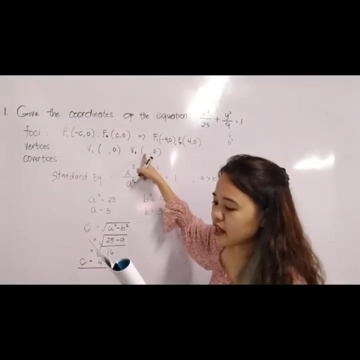 a okay, read again, or please watch again our last video in order to review our definition of the vertices, or please, please, okay. so since this is negative x and positive x, so negative or positive x, which is equal to okay, so for the vertices, x equals positive or negative. 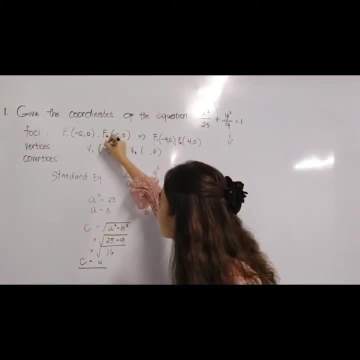 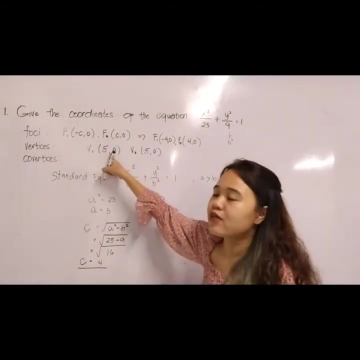 a, so this is 5, okay, and negative 5. so positive 5 and negative 5, okay. then what do you call a, a or c vertices? this is it for the vertices. let's have variable a. for the co-vertices, let's have: 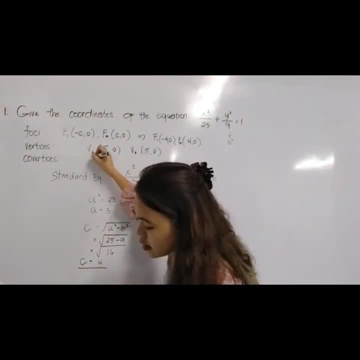 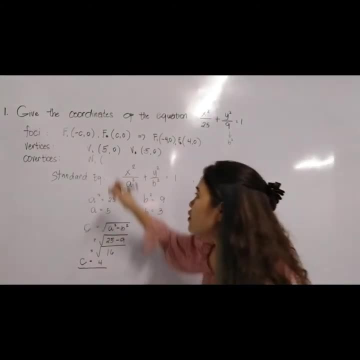 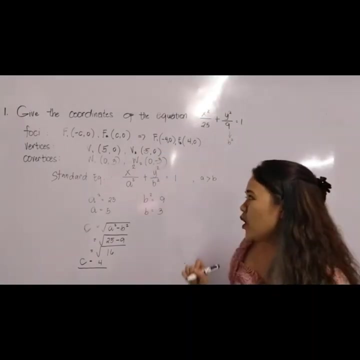 variable b. okay, so for the co-vertices, we have w as our variable. w we have, if our value of x is 0, then the co-vertices is positive 3 or the co-vertices is negative 3. okay, so again, this is for the foci. 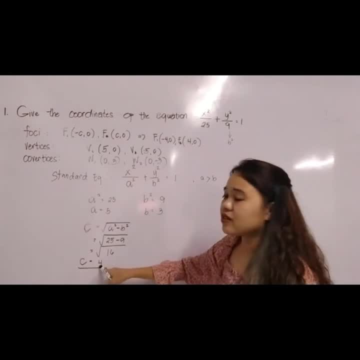 you just have to remember you will be using the variable c that we saw. for the vertices, we will be using the variable a that we got earlier, and for the co-vertices, we will be using the variable b. okay, so this is on how to find the coordinates. 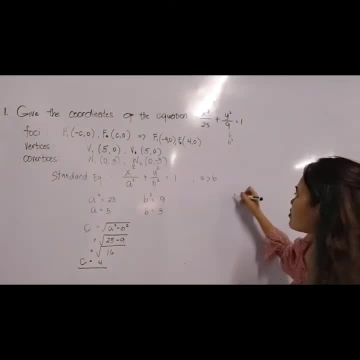 now let's graph. let's proceed to the graph. if this is our partition plane, okay. so this is our center. 0. we have 1, 2, 3, 4. 1, 2, 3, 4- okay. negative cell host and. 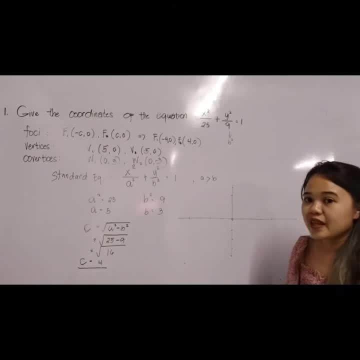 this is the left side. okay, so we have the center at 0, we have the foci negative 4, 4, 0. negative 4, 0, this one here, our foci 4, 0 here. okay, this is f2. 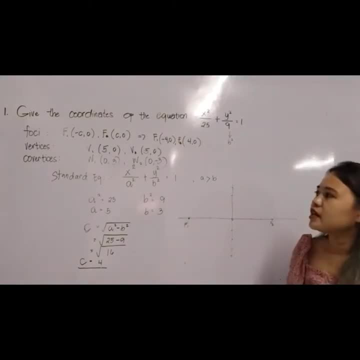 and this is f1. now let's have the vertices. we have 5, 0 and negative 5, 0, so negative 4, we have negative 5 and we have positive 5. so this is the vertices. so this is v1 and v2. 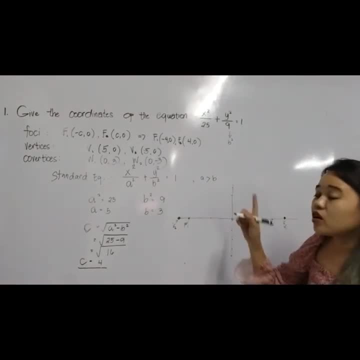 okay, now let's have our co-vertices. so co-vertices is in the y-axis, it's 0, 3 and 0, negative 3. this is 3 and negative 3. okay, so our points are complete, which we can use in order to form. 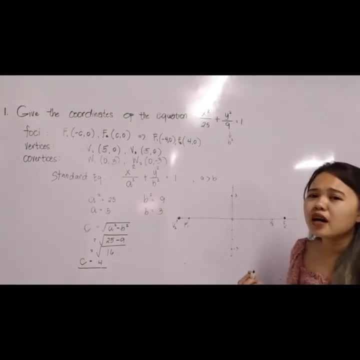 our graph. make sure if- um, I have seen some of the outputs last school year so I want to take one round straight line, okay, then we can form an ellipse. so make sure an ellipse is formed in um connecting our points. so, in connecting our points, then therefore we have 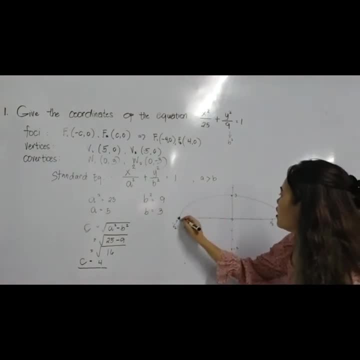 okay, sorry kayo if it's not okay. perfect ellipse, okay. so therefore, this is our graph, so it's ellipse, guys, um, um, okay. so again, make sure that in graphing the ellipse it's straight line connecting our points. okay, so this is our first example on how 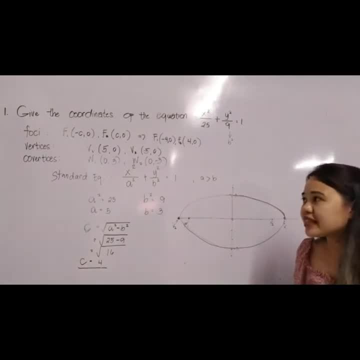 to find the coordinates for the posi vertices and co-vertices. I hope you understand, thank you.